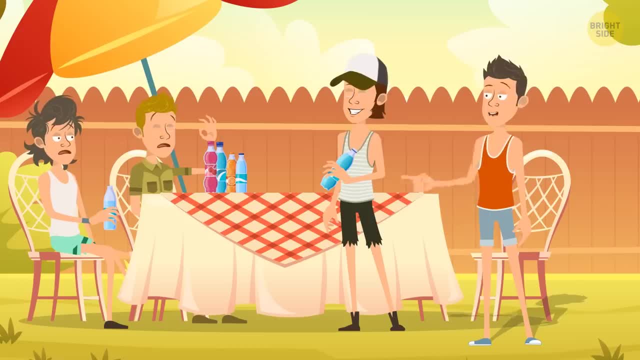 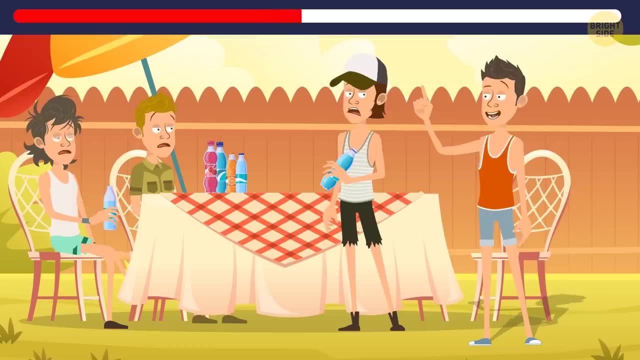 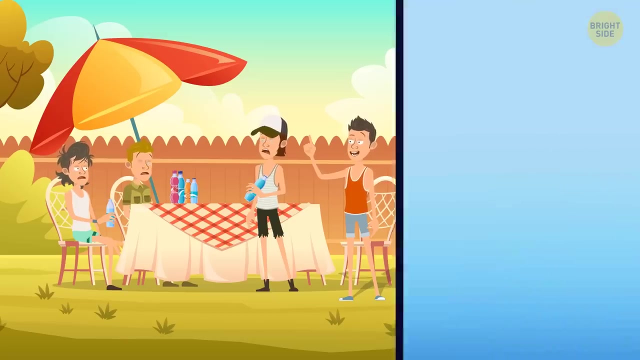 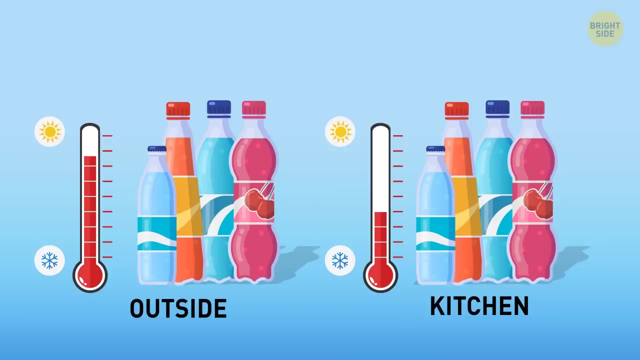 but one of them cut in. You were cheating, he said. Why did he think so? It was an extremely hot day. No wonder the water had been outside for several hours, which was much warmer than the water brought from the kitchen. Someone robbed a bank in a large city. A police detective went to visit the main suspect. 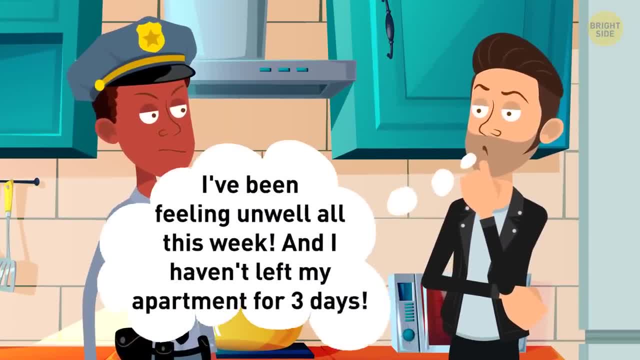 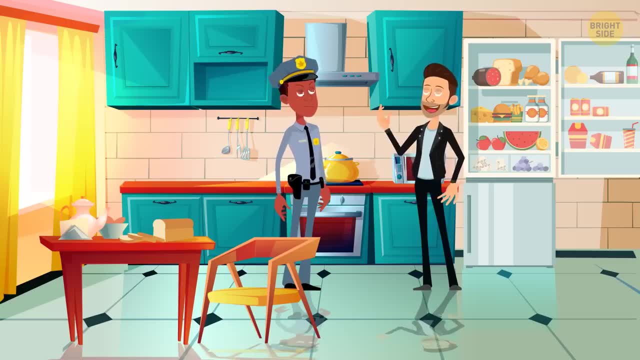 who had been detained several times before. I've been feeling unwell this week and I haven't left my apartment for three days. Luckily, I didn't need food. My fridge is full, You can make sure of it yourself. the man said and opened his fridge, But the detective realized the man was lying. 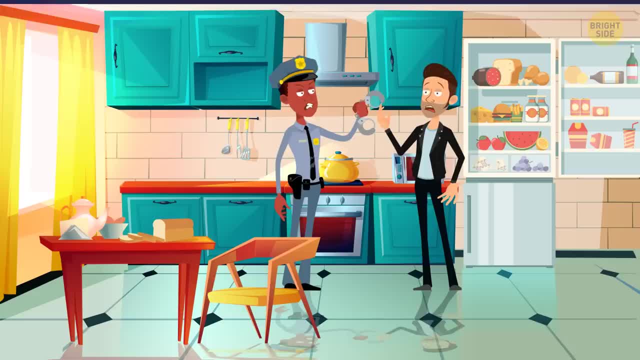 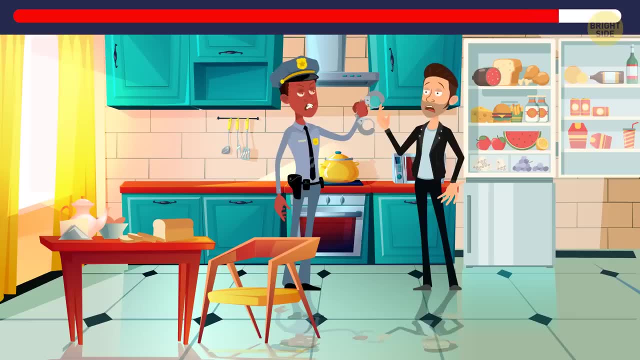 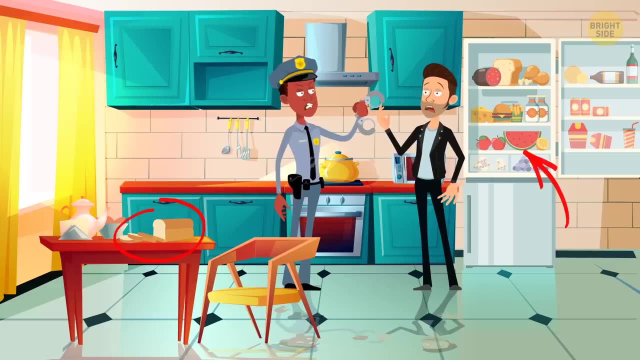 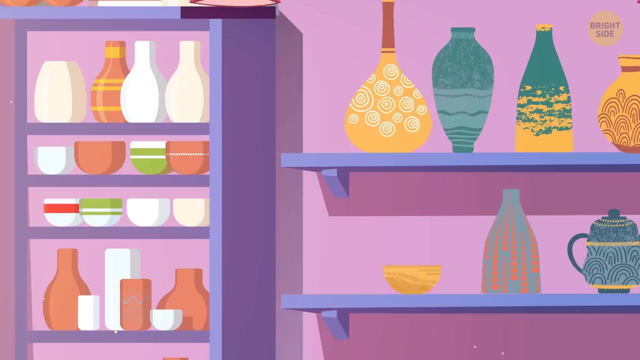 and arrested him. How did he figure it out? First of all, that loaf of bread on the table looks fresh. Plus, if the man had been staying inside for three days already, his fridge wouldn't be so full. Mr Black sold beautiful, rare vases. There were dozens of them on the shelves of his store. 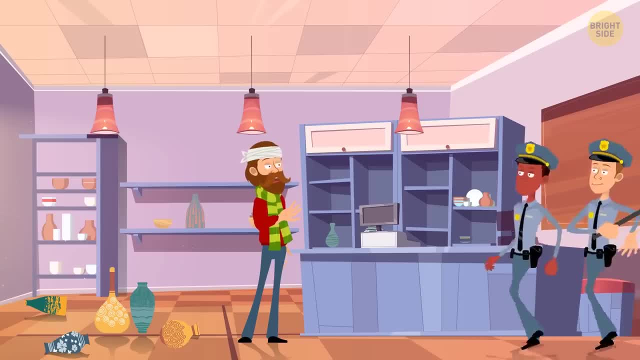 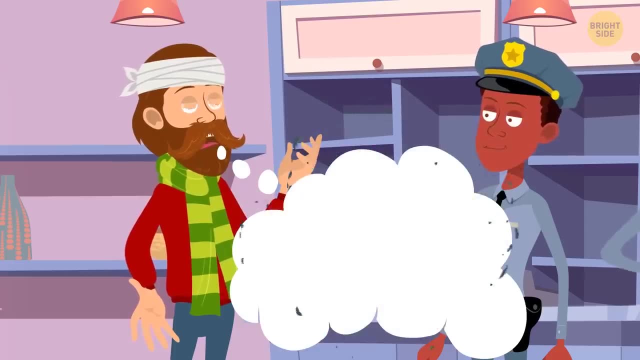 One day the man called the police. When they arrived, the owner had his head bandaged and his store was a mess. Some guys in masks ran into my store and grabbed the money and the most expensive vases. Then they hit me on the head and I blacked out. 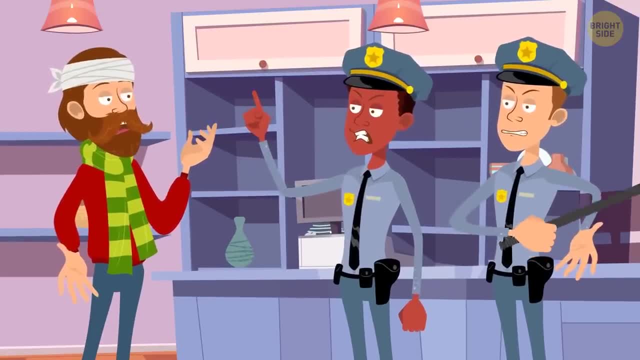 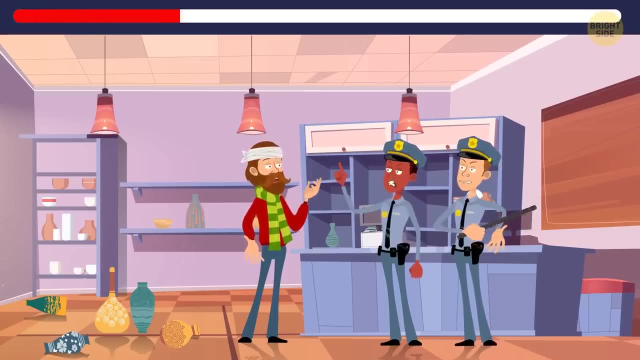 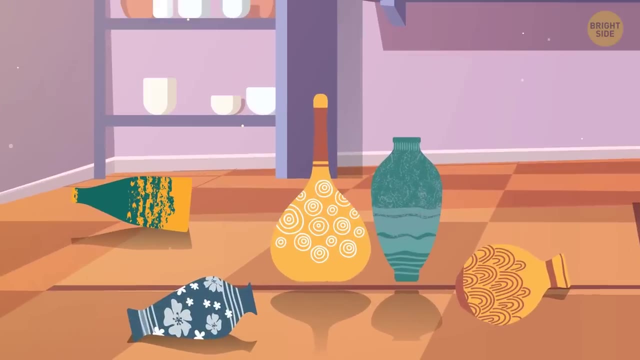 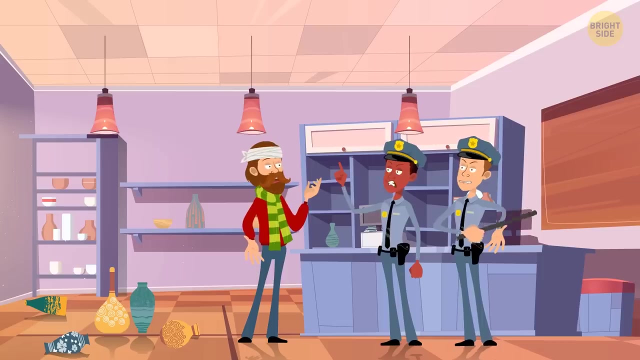 Police officers immediately understood that Mr Black was lying to get the insurance money. How did they figure it out? Even though most of the vases are on the floor? they aren't even cracked. But if the vases had fallen down from the shelves during the robbery they would have been shattered. 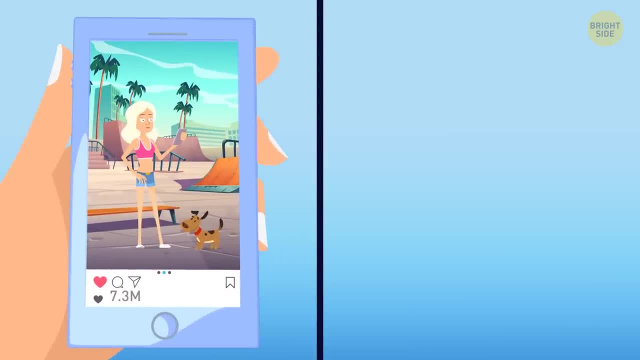 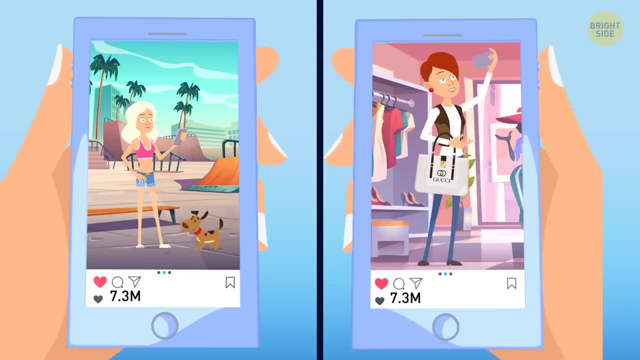 Look at these two bloggers, As you see. they both seem to be very popular. They also have the same amount of likes, But there's something wrong with one of them. She must be hiding something. What is it? The girl on the right has a fake bag. 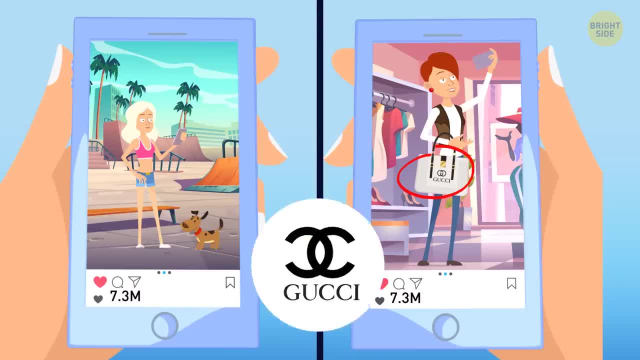 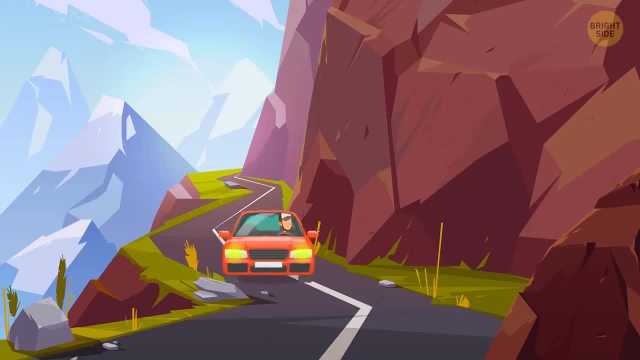 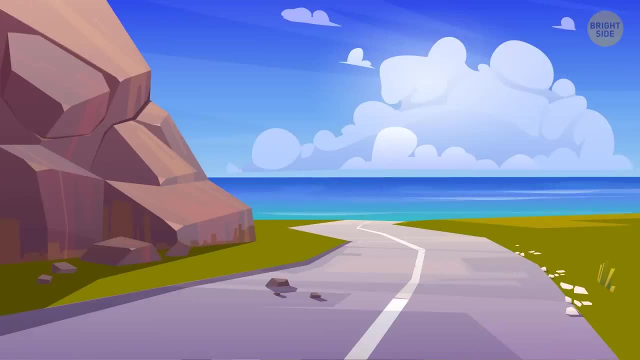 The logo on it looks like that of Chanel, but it's written Gucci underneath. Marcel was driving along a dangerous mountain road. Suddenly he saw a man sitting on the side of the road and stopped. It turned out the man hadn't managed to control his car. 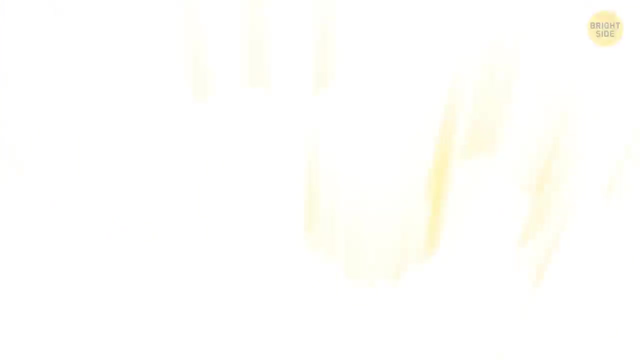 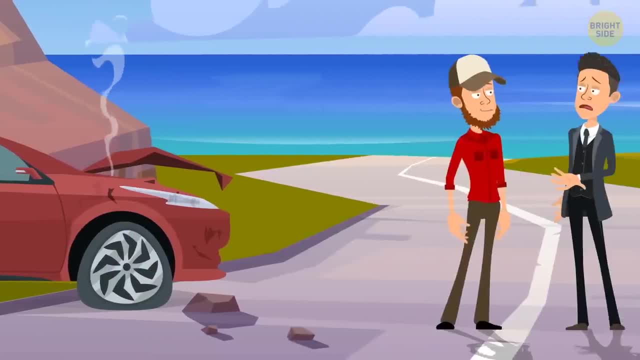 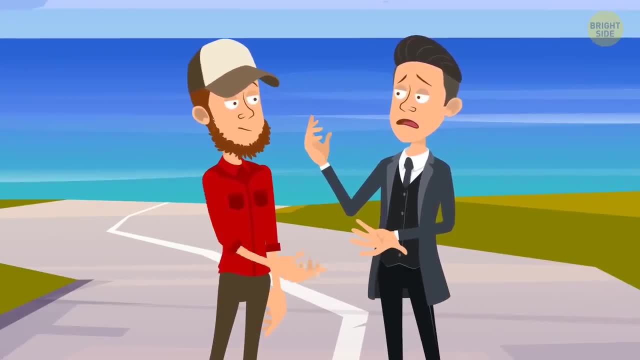 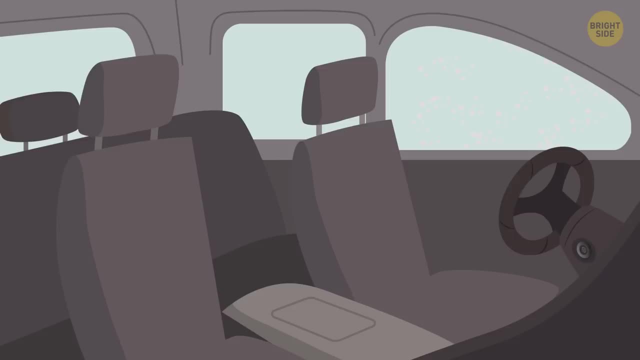 The man asked Marcel. The guy agreed but asked the man to show him what was inside the car. The man took the key out of his pocket and unlocked the damaged vehicle. I won't take part in this fraud, Marcel said. Why did he think the man was lying? 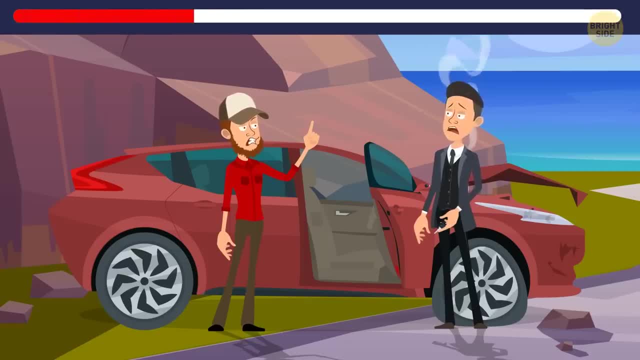 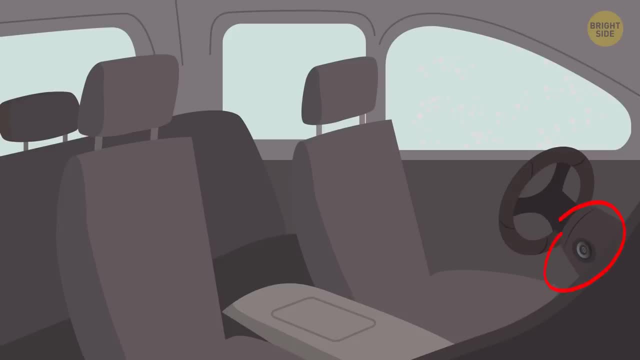 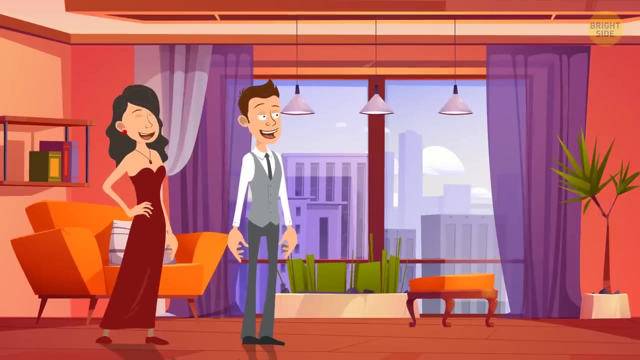 I won't take part in this fraud. Marcel said I won't take part in this fraud. Marcel said If the man had been thrown out of the car, the key would still be in the ignition. Dylan and Susan had been happily married for 10 years. 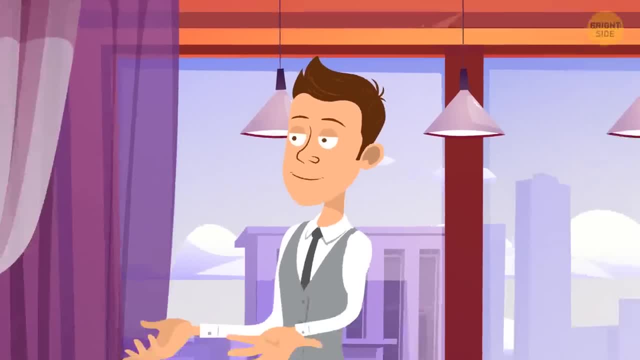 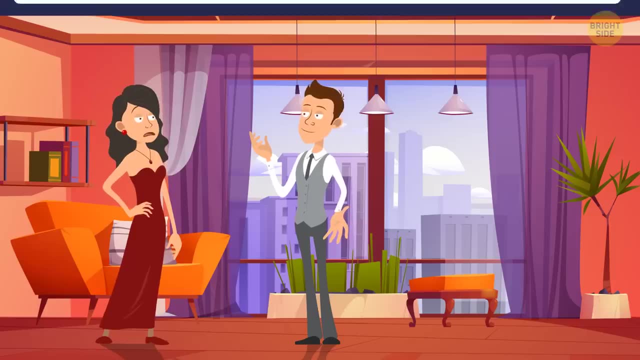 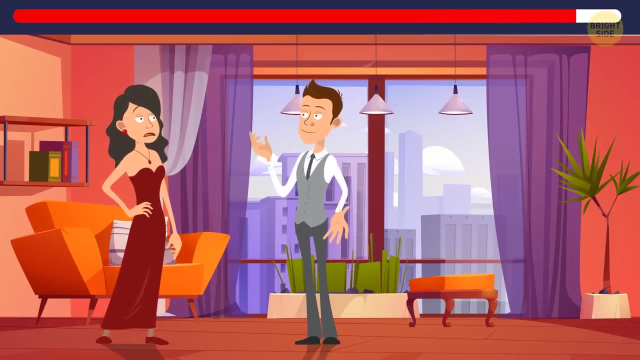 One day Dylan went on a business trip. When he returned, Susan immediately understood that the man wasn't her husband. How did she figure it out? Dylan always wore his wedding ring. If you were attentive, you must have noticed it on his finger. 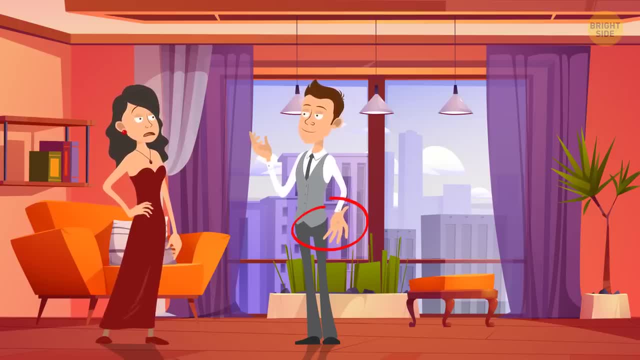 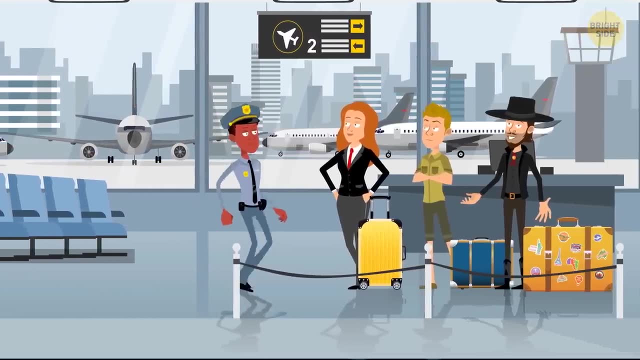 But the man who returned to Susan didn't have the wedding ring. The police found out that a smuggler was going to leave the country through the largest airport in the city. A detective arrived there and detained three people who looked like they were married. 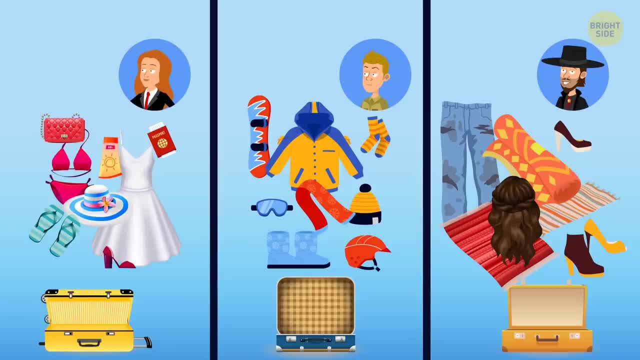 They looked suspicious. Look at them and try to figure out who the smuggler is. It's the third passenger. His suitcase is full of totally random stuff: Women's shoes, some random socks, a pair of old dirty jeans and even a wig. 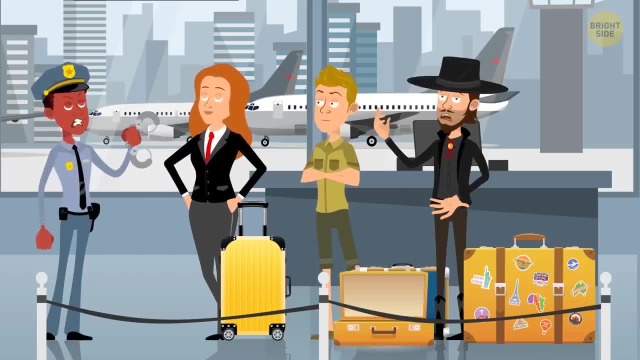 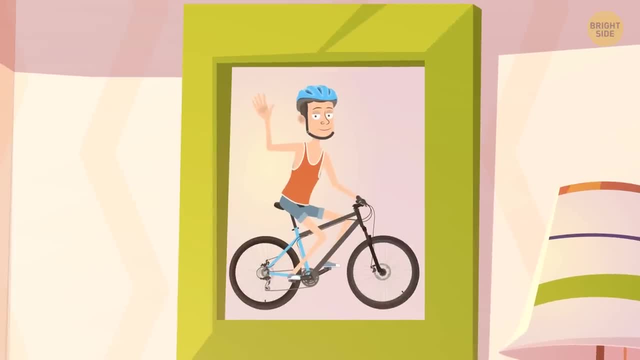 Plus, when closed, the suitcase looks much larger than when it's open. Sarah's husband, Michel, was a professional cyclist. He was about to have a challenging cycling tournament. I promise I'll bring you the bouquet they give to the winner. Michel told Sarah. 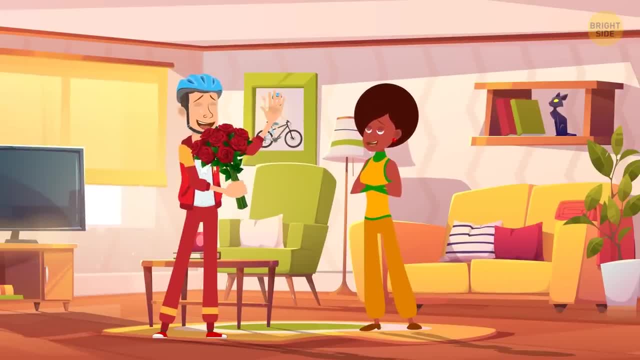 Four hours later he came back with beautiful flowers, But Sarah realized right away that Michel hadn't won the tournament. How did she figure it out? His wife Catherine said the same thing. She said These flowers are actually from Sarah's garden. 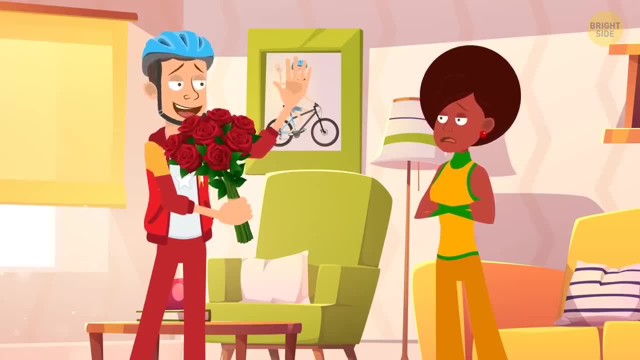 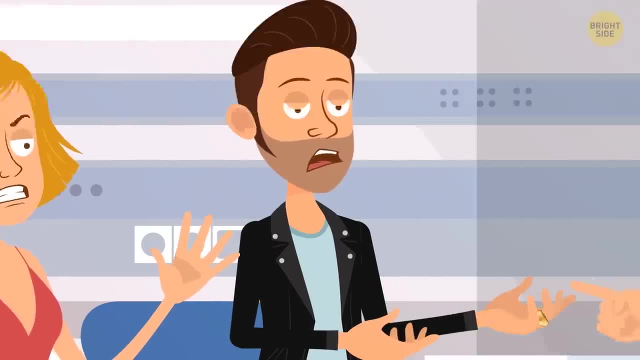 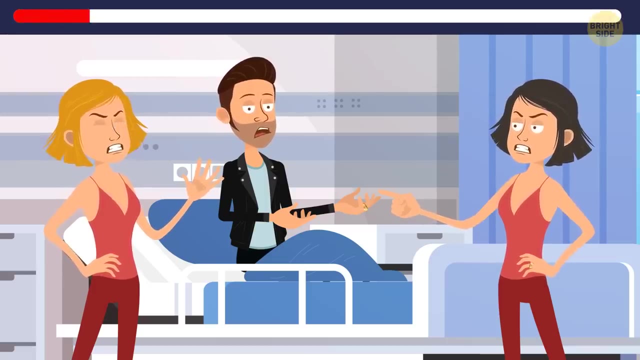 The same flowers are growing next to their house. Look at these people. The man is in the hospital. He's lost his memory And these two women both claim to be his partner. One of them is obviously lying, But which one? The woman on the left is lying? 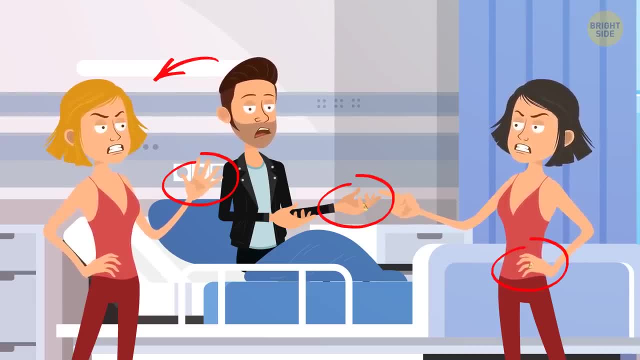 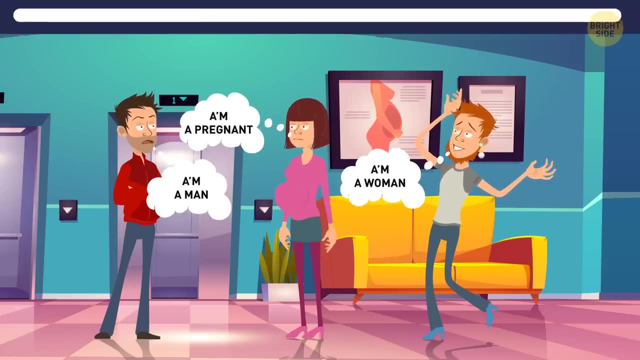 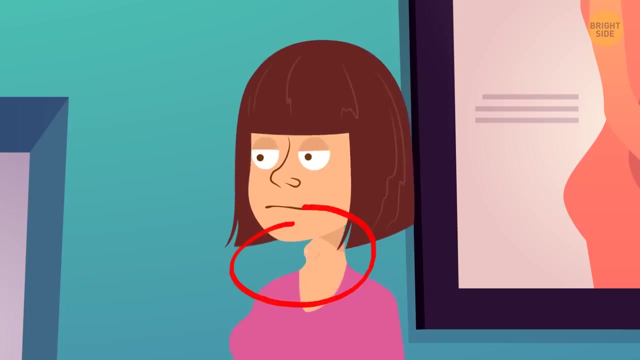 If they were married, they would have wedding rings on their fingers. Now there are these three people. One of them is lying. Who is it? Look at this woman claiming that she's pregnant. See that Adam's apple. It's a man. He can't be pregnant. 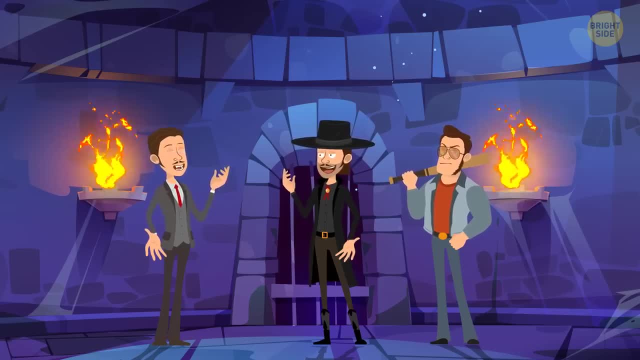 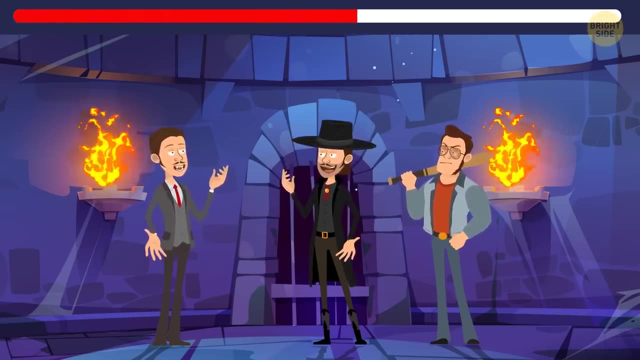 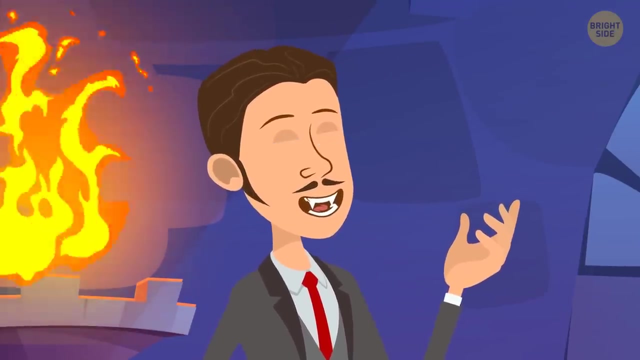 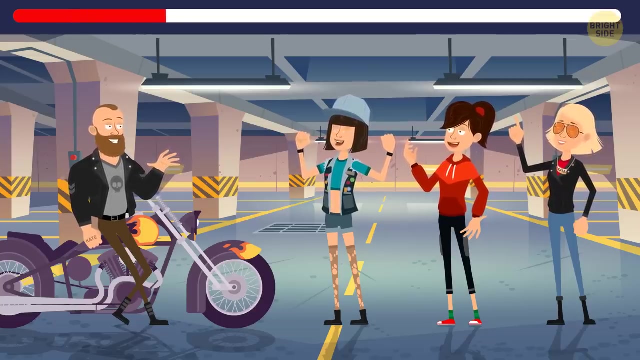 Look at these people. Can you figure out who's a vampire? It's this man. See those fangs Creepy. Which of these girls is the man's wife? It's the girl on the right. She's wearing a necklace saying Kate, And the man has a tattoo with the same name on his arm. 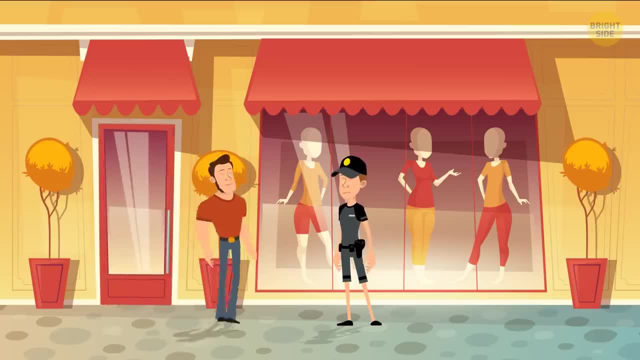 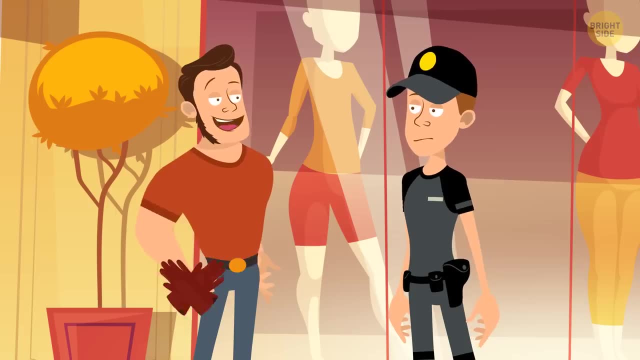 A store security guard stopped a man who was leaving a clothing store. The sales assistant claims: you've stolen a pair of expensive gloves. These are my gloves. I've had them for ages. But the security guard immediately says He immediately understood the man was lying, How The man wouldn't be able to use these gloves.